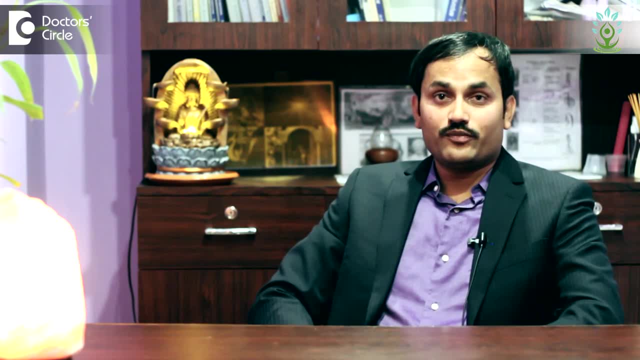 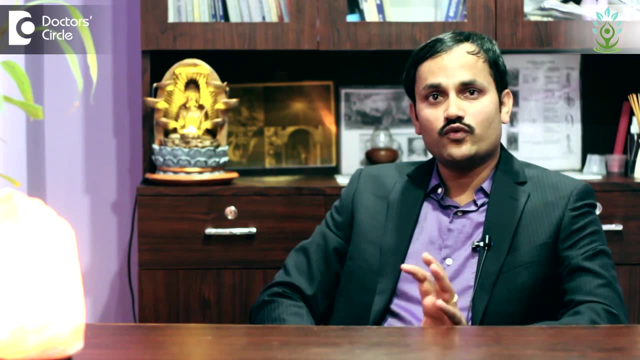 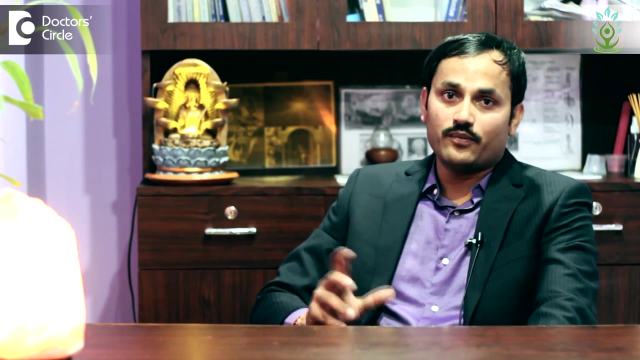 different asanas, in that very difficult to find the five top more asanas, But still I can able to give you the five beneficial asanas which you can do very easily. The first one is the Sirs Asana. as this name, Sirs, means the top Sirs Asana. 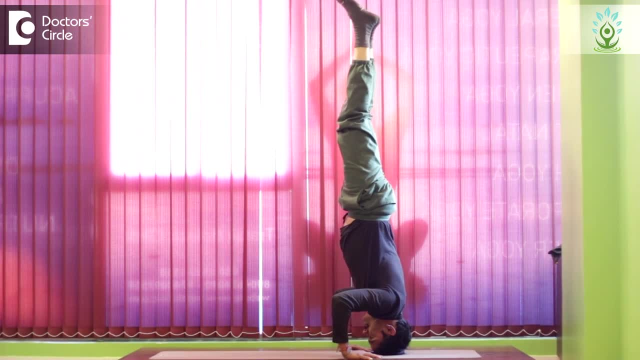 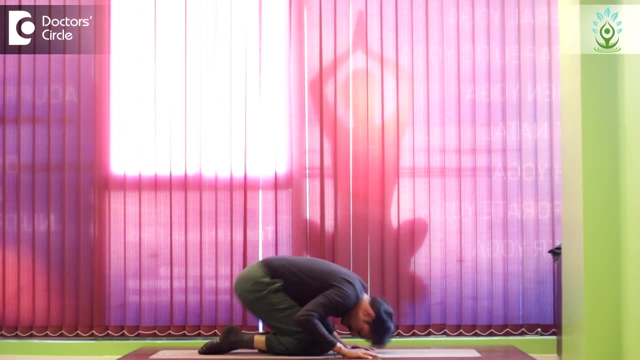 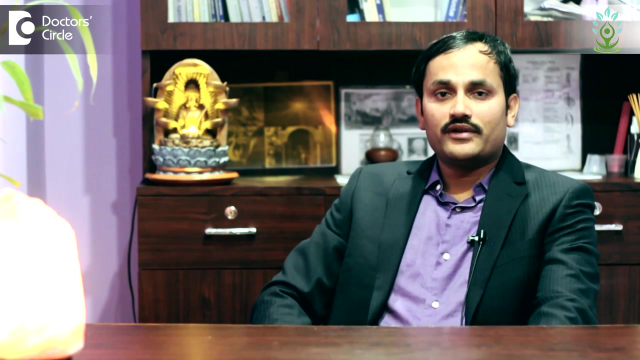 In that pose you have to do the head down and legs up. This is the one of the best asanas for all the endocrine glands, especially the pituitary, the thyroid, the all the other glands. It is good for the thyroid problem. 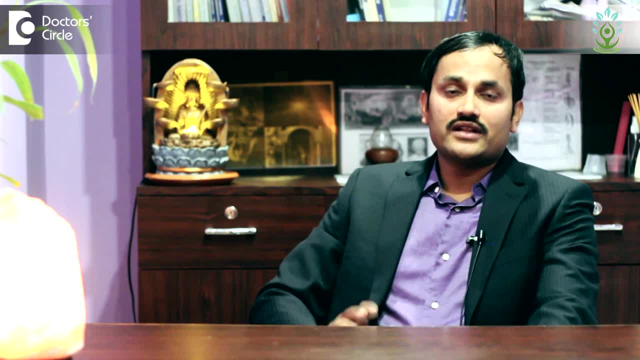 It is good for the concentration problem, It is good in the insomnia and it is very good asanas to varicose vein and different different problem. There is some limitations of this asanas: The person who has a high BP, the person who has a heart problem, the cervical problem. 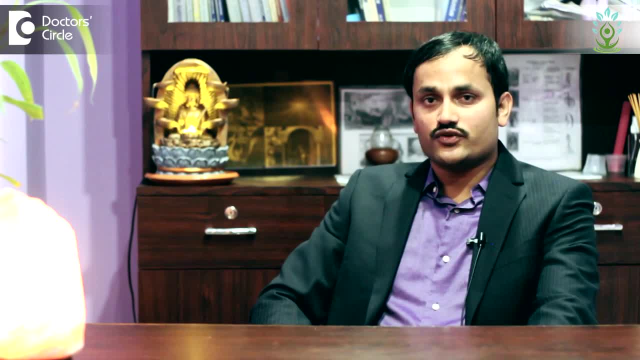 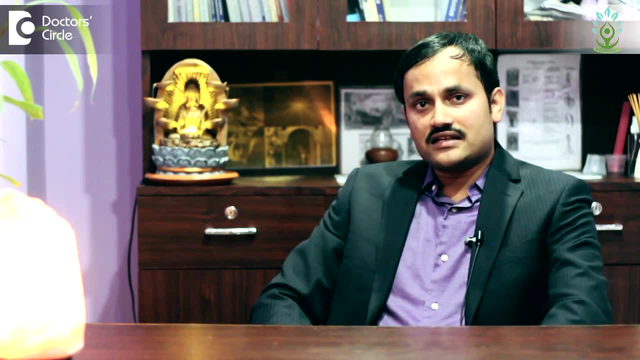 should not do this. asanas: After the Sirs Asana: you have to relax in the any comfort Comfortable asanas like a Sasankasana, Vajrasana, Sasankasana and any rabbit pose: you have to relax. 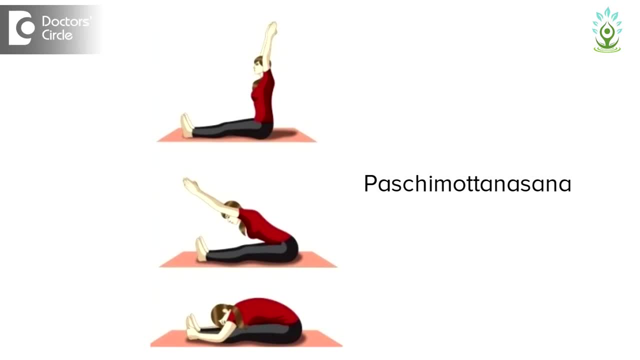 The next asana is the Paschimuttanasana. as this name, Paschimuttanasana, This means that your back part will get a stretch once you are doing this asanas. So in this, this asana is very good for the teenagers as they have an immense energy in. 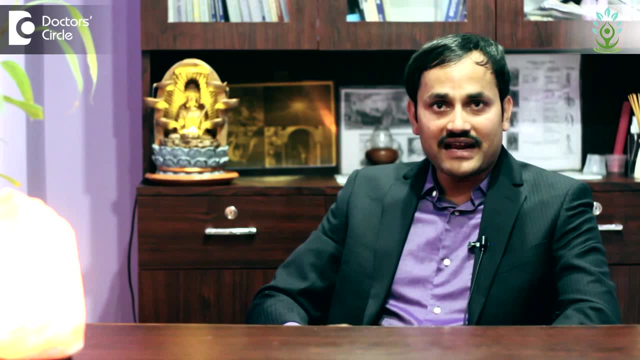 their Mooladhara and Swadhisthana Chakra. Once they will practice this asanas, This asana, It will improve their concentration. good for the flexibility of the back, good for the calf muscles, good for the hamstring. This is the one of the best asanas. 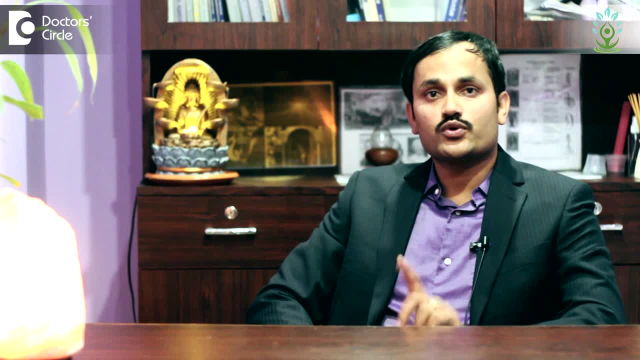 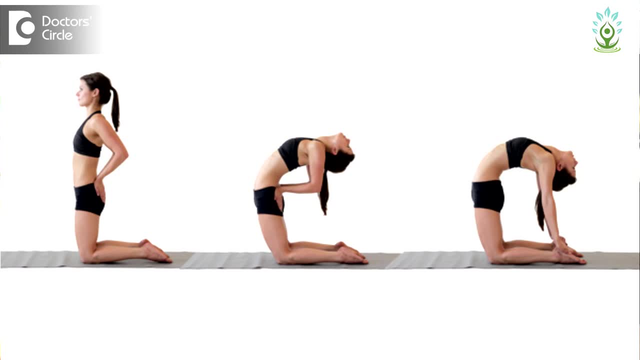 The complementary asana of the Paschimuttanasana is Uroostasana. So Uroostasana means camel pose, Camel pose. You have to catch the heel at the back. The benefit of this: camel pose is very good for the kidney, very good for the heart muscles. 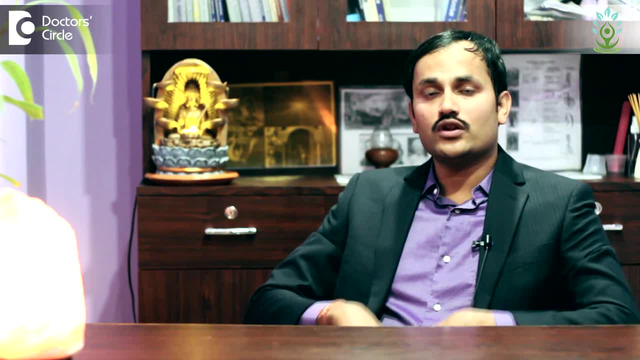 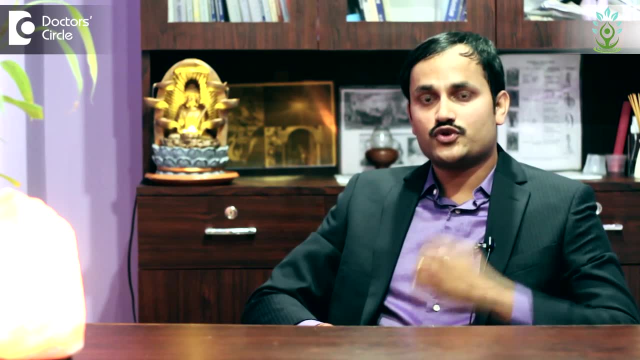 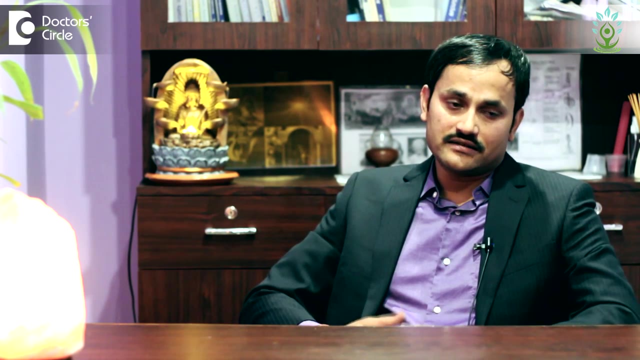 good for the shoulder And very good for the all the genital organs, Good for our digestive system. After the Uroostasana you have to do any asana which is the forward bending asanas, like a Yoga Mudra and any forward bending asana.